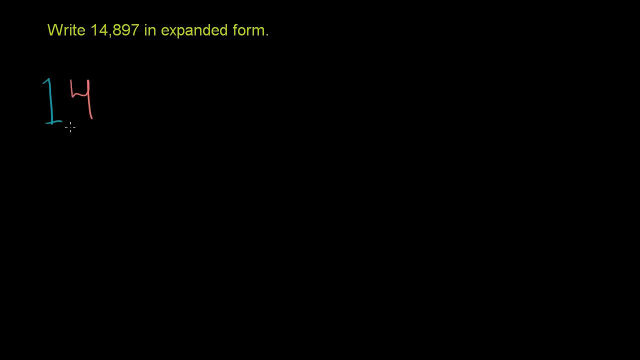 14,800 and 97.. See, I already used the blue. Maybe I should use yellow And 97 in expanded form. So let's think about what place each of these digits are in This right here. the 7, is in the ones place. 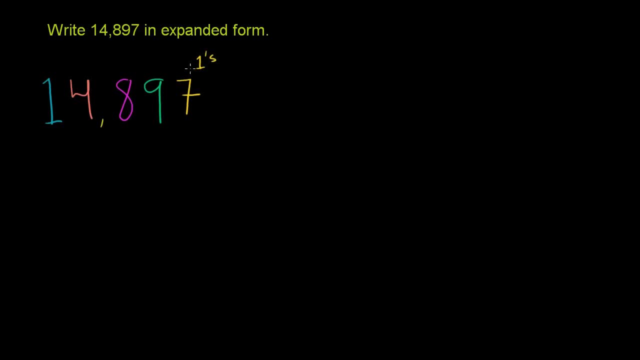 This is in the ones place. This is in the ones place. The 9 is in the tens place. This literally represents nine tens, and we're going to see this in a second. This literally represents seven ones. The 8 is in the hundreds place. 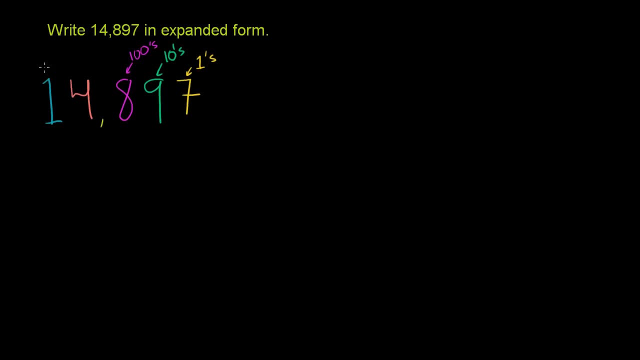 This is in the hundreds place. The 4 is in the thousands place. It literally represents 4,000.. So this is in the thousands place And then the 1 is in the tens thousands place. And you see, every time you move to the left, you move one place to the left, you're multiplying. 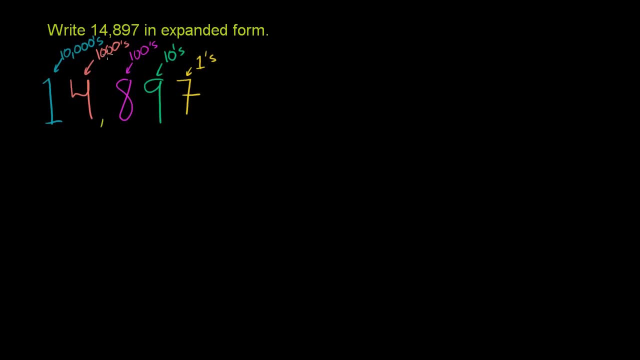 by 10.. Ones place tens place. hundreds place. thousands place tens thousands place. Now let's think about what that really means. If this 1 is in the tens thousands place, that means that it literally means it literally represents. so this 1 literally represents. I want to do this in a way that my arrows 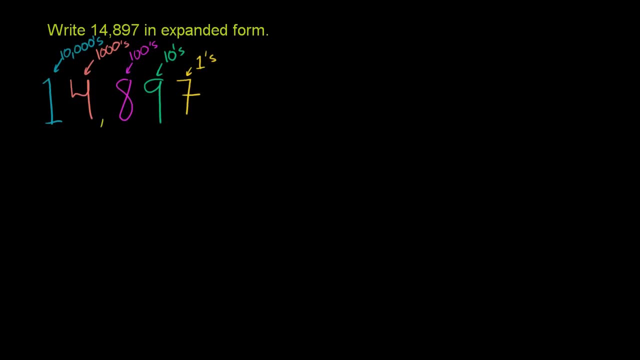 don't get mixed up. Actually, let me start at the other end. Let me start with the 7 represents. The 7 literally represents seven ones, Or another way to think about it. it also you could say it represents seven times one. 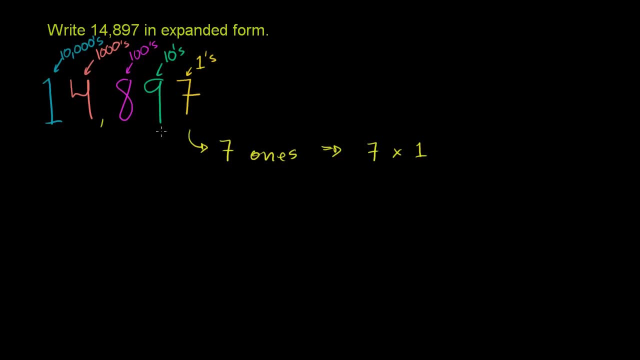 All of these are equivalent. It represents seven ones. Now let's think about the 9.. That's why I'm doing it from the right, so that the arrows don't have to cross each other. So what does the 9 represent? 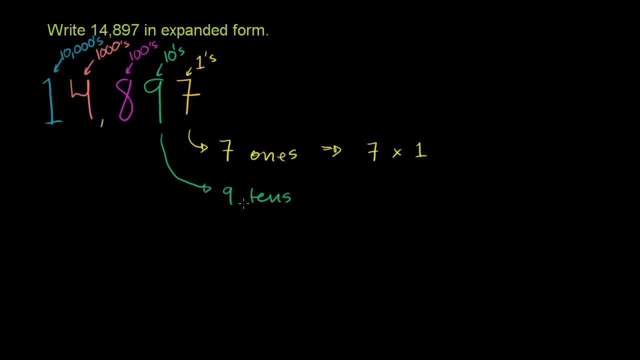 It represents nine tens. You could literally imagine you have nine actual tens. You could have a 10 plus a 10. Plus a 10. Plus a 10. Do that nine times. That's literally what it represents: Nine actual tens. 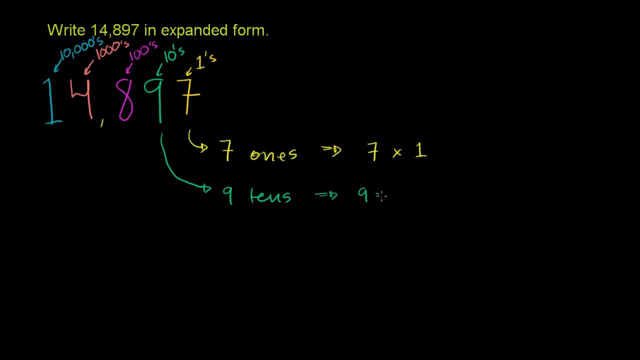 Nine tens. Or you could say it's the same thing as nine times ten. Or 90. Either way, you want to think about it, So let me write all the different ways to think about it. Or 90. It represents all of these things. 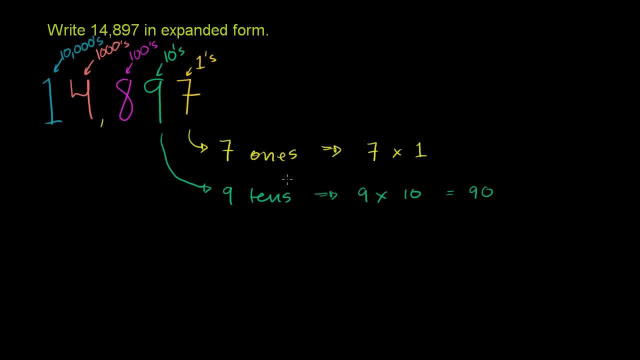 Nine tens, or nine times ten, or 90.. So then we have our 8.. Our 8 represents- We see it's in the hundreds place- It represents eight hundreds, Or you could view that as being equivalent to 8 times 100.. 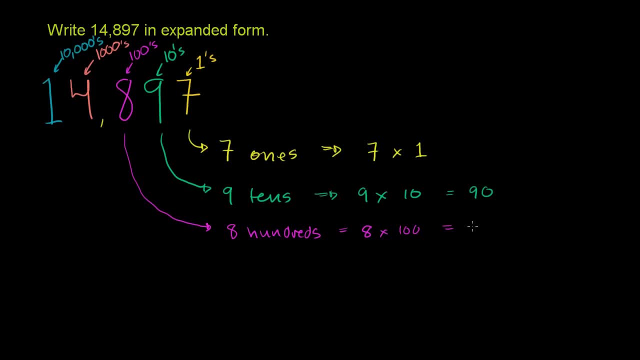 A hundred, not a thousand. Eight times a hundred Or eight hundred, That 8 literally represents eight hundreds, And then the 4. I think you get the idea here. This represents in the thousands place. It represents four thousands, Four thousands. 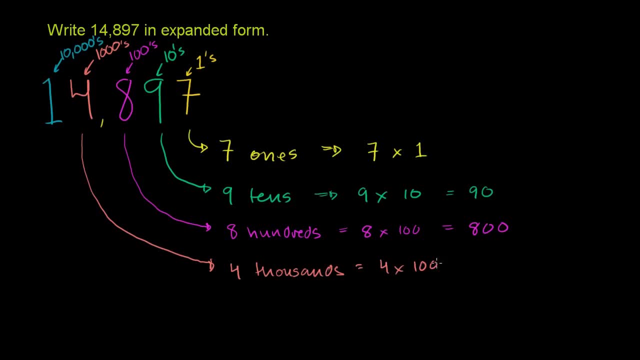 Which is the same thing As four times one thousand, Which is the same thing as four thousand. Four thousand is the same thing as four thousands added up. And then, finally, we have this one Which is sitting in the ten thousands place, So it literally represents one ten thousand. 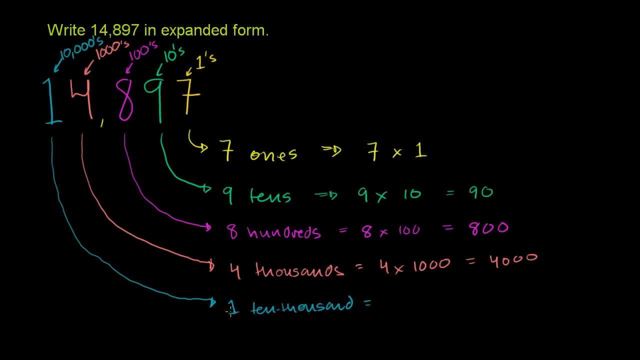 Or you could imagine it. You could imagine if these were kind of chips, Kind of poker chips. That would represent A blue poker chip And each blue poker chip represents ten thousand. I don't know if that helps you or not. And one ten thousand is the same thing as one times ten thousand. 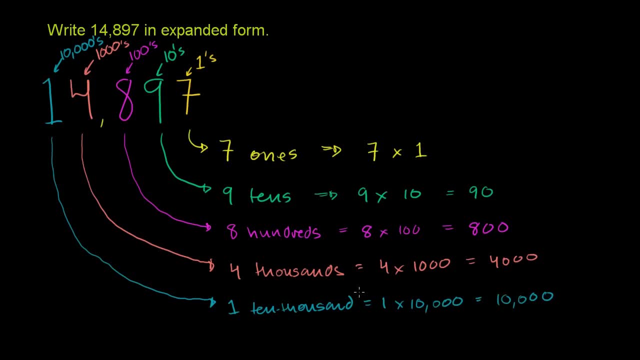 Which is the same thing as ten thousand. So when they ask us to write it in an expanded form, We could write 14,897 literally as the sum of these numbers Of kind, of its components, Or we could write it as the sum of these numbers. 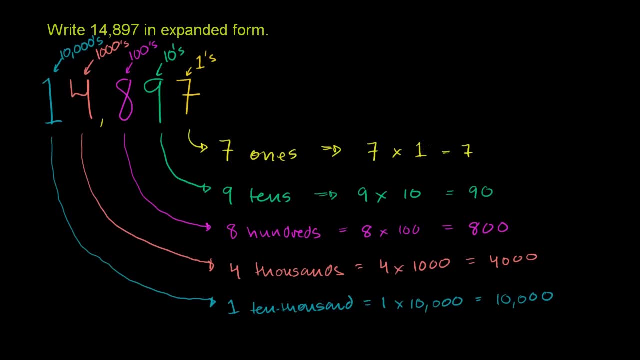 Actually let me write this: This top seven times one is just equal to seven. So 14,897 is the same thing As ten thousand plus four thousand plus eight hundred plus ninety plus seven. So you could consider this expanded form Or you could use this version of it. 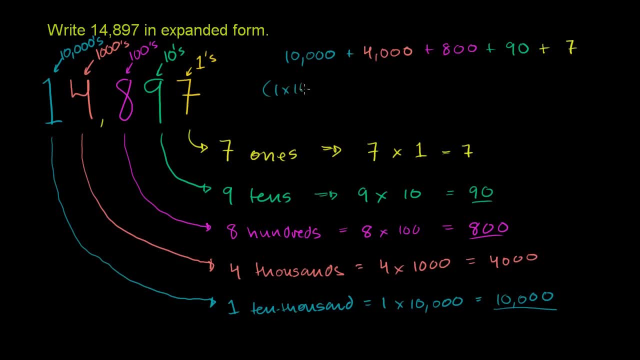 You could say this is the same thing as one times ten thousand- Depending on what people consider it to be expanded form- Plus four times one thousand, Plus eight times one hundred, Plus nine times ten Plus seven times one. Scroll to the right a little bit.